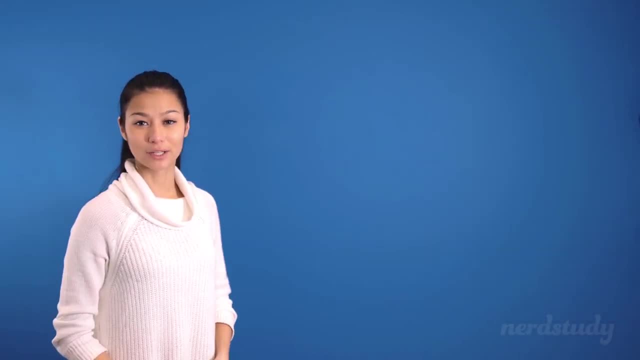 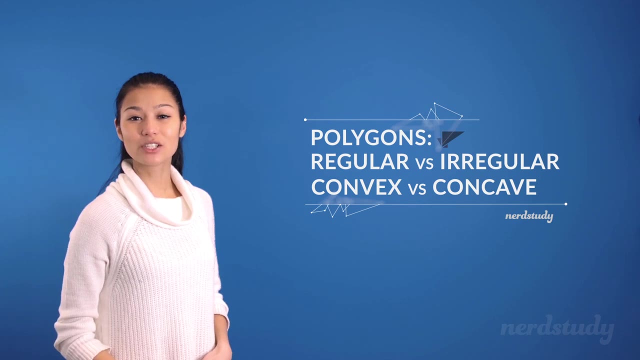 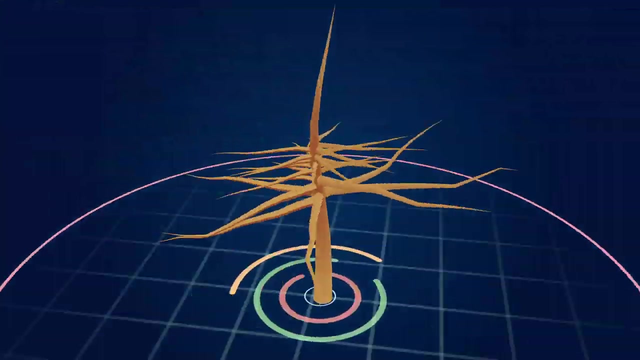 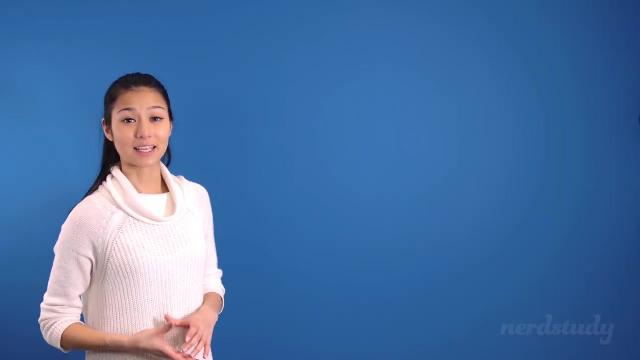 What are polygons and what makes them regular or irregular? Also, what makes them convex or concave? In this video let's dive into an introduction of the 2D world of polygons. So let's begin with an example of a polygon here. 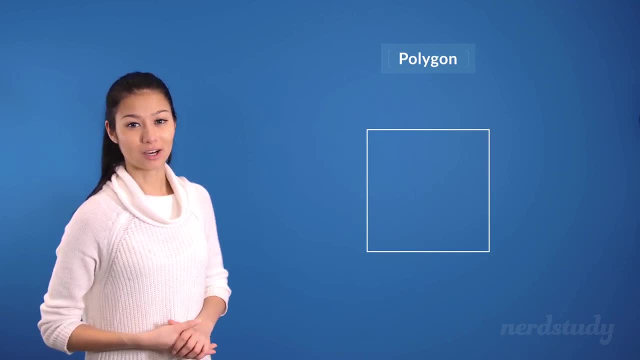 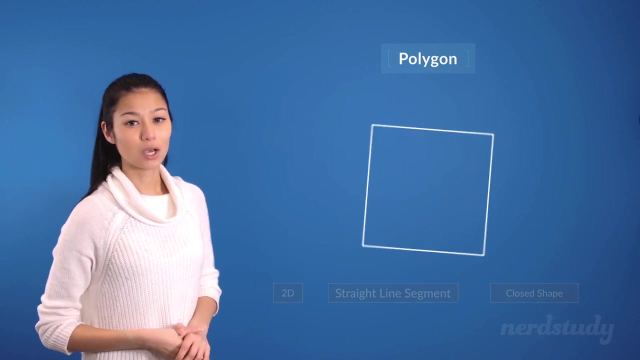 Now, what are the characteristics of a polygon? Well, a polygon is a two-dimensional shape that is made up with straight line segments, which means absolutely no curves. The shape for a polygon is always a closed shape. So, while this shape over here is two-dimensional that's made up of straight lines, 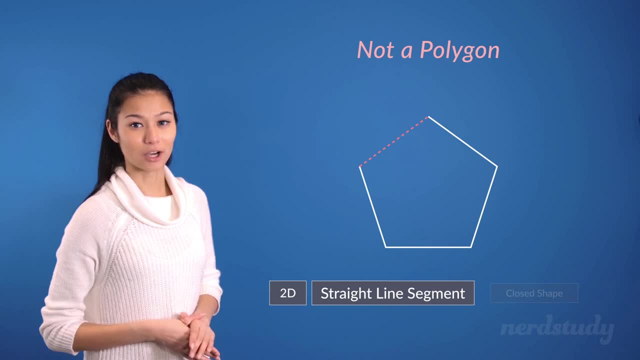 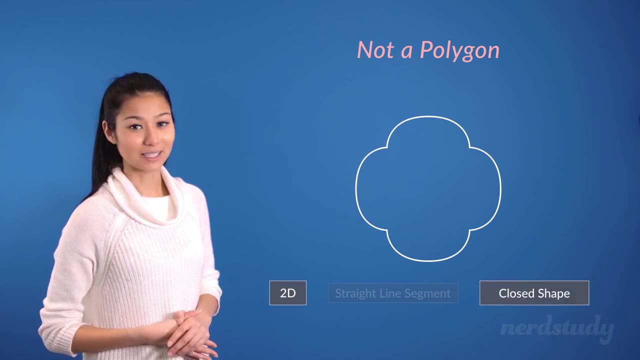 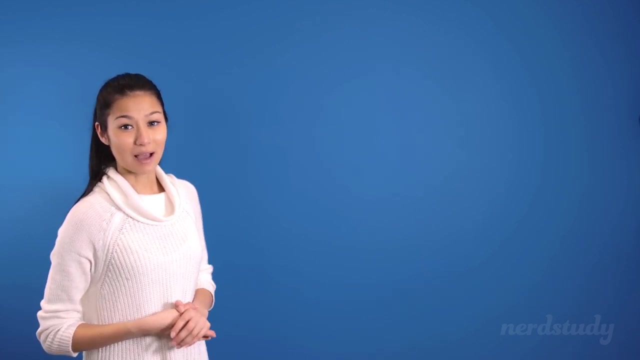 since it does not close up, it is not considered a polygon. Also, while this unique looking shape is made up of straight lines, it is not considered a polygon either, since its edges are not straight lines, but rather curved Awesome. So if we were asked if a real-life basketball was a polygon or not, what would our answer be? 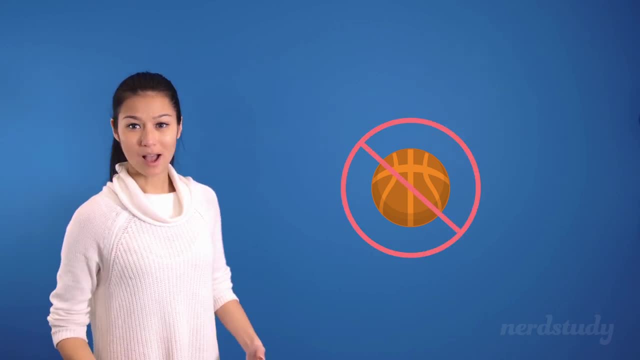 Well, the answer to that would be no. And why? Well, the reason relates to the fact that a ball is made up of straight lines. The reason relates to the fact that a ball is made up of straight lines. The reason relates to the fact that a ball is made up of straight lines. 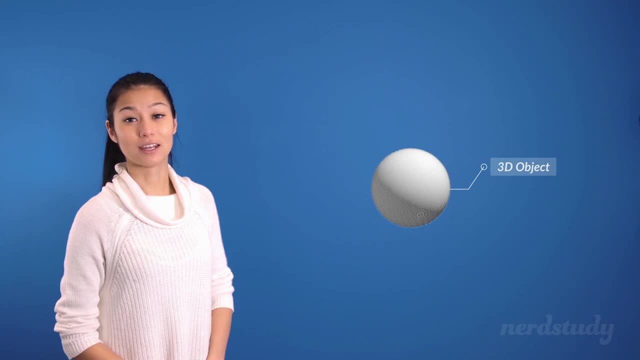 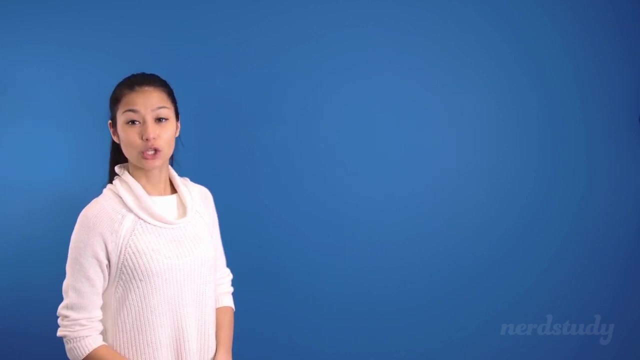 The reason relates to the fact that a basketball is a three-dimensional object rather than a two-dimensional shape, which is one of the criteria for a shape being a polygon. Great. So, moving on with more information about polygons, we can actually categorize them into two categories, which are regular versus irregular polygons. 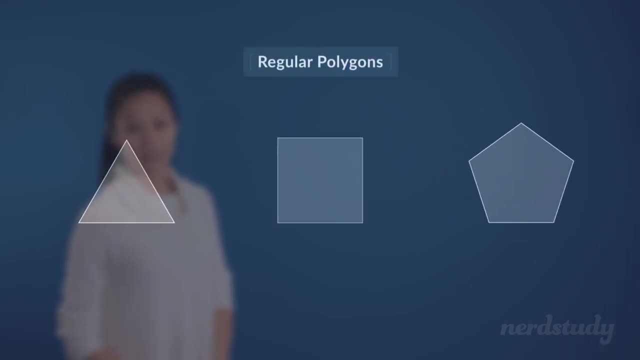 So the following are examples of regular polygons. Now, if we look carefully at these polygons, we'll notice that each of these sides are equal to every other side in the polygon And as a result of that, we've got equal angles on the insides as well. 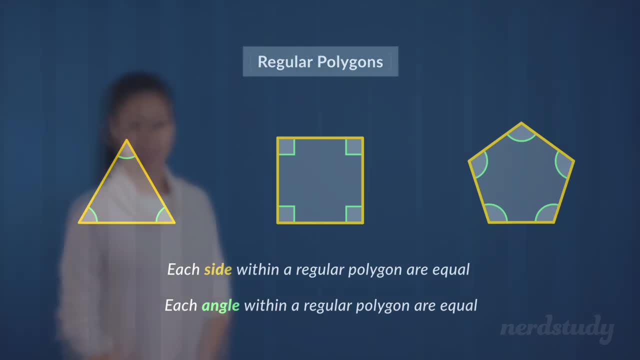 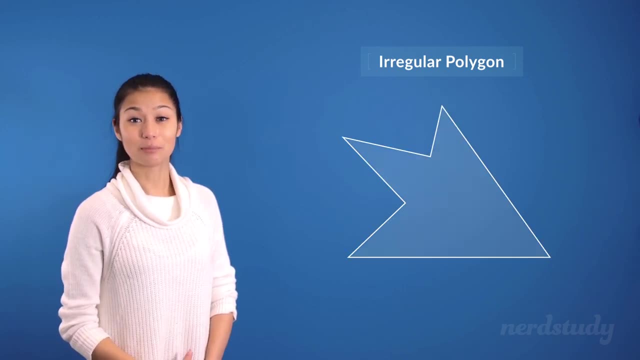 This is what makes a polygon a regular polygon. As for an irregular polygon, if we take a look at this funny-looking shape here, we would still call it a polygon, since it is made up of line segments and it's a closed object. 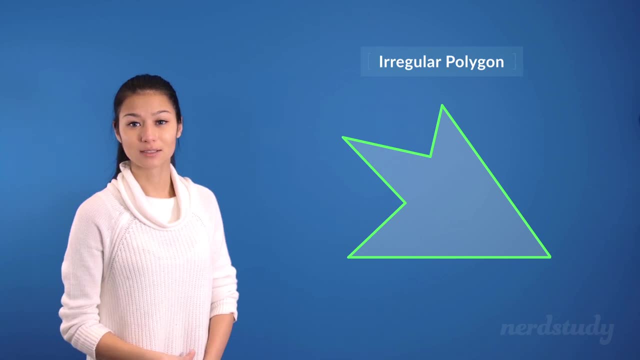 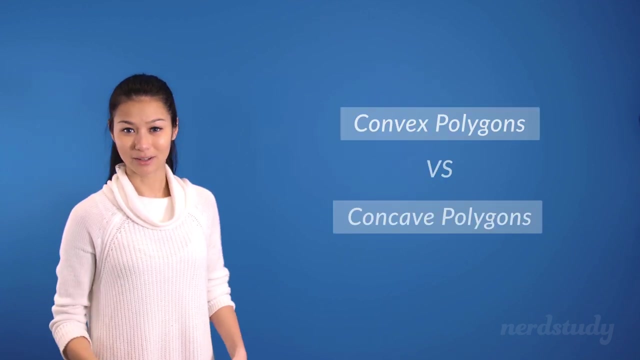 But we wouldn't be able to call it a regular polygon, since the line lengths aren't all the same And obviously not all the angles are the same as well. All right, and now, to finish off this video, let's talk about convex polygons and concave polygons. 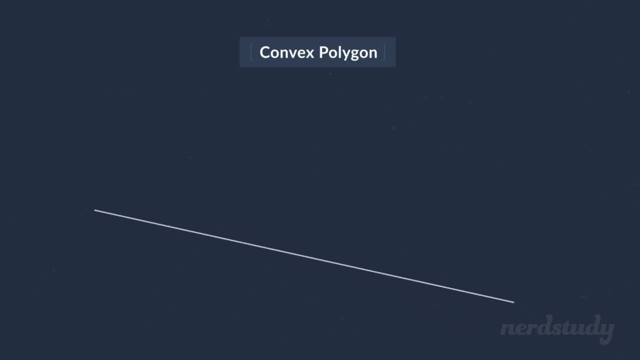 An example of a convex polygon might look like this. Now notice how all of the angles on the inside are less than 100. So the differentiating characteristics of a convex polygon is that each angle within the polygon must be less than or equal to, 180 degrees. 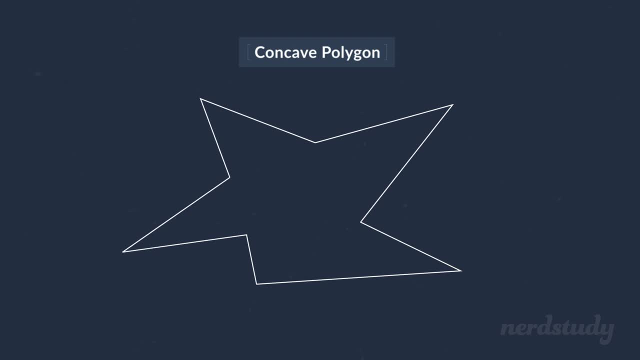 A concave polygon, on the other hand, has at least one angle on the inside of the shape that is greater than 180 degrees. This shape, for example, which also happens to be irregular, is a concave polygon. It's irregular because, clearly, not all side lengths are equal to each other. 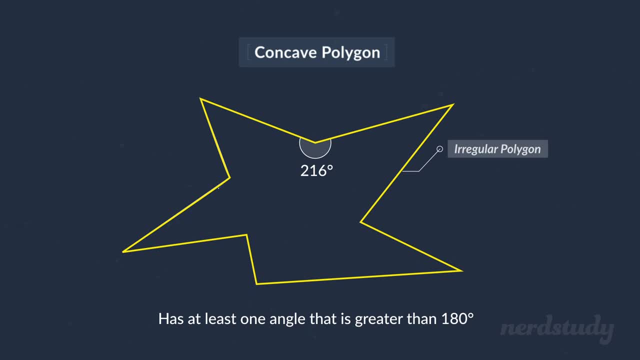 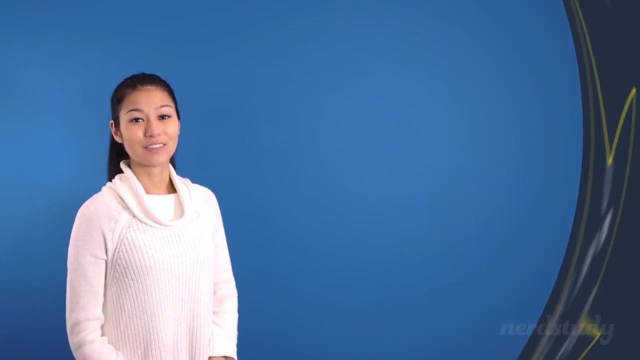 And it's concave, since not all angles on the inside are under 180 degrees, For example. this angle right here is clearly greater than 180 degrees. Awesome. So that's the end of this lesson on polygons and the different types of polygons we can come across. 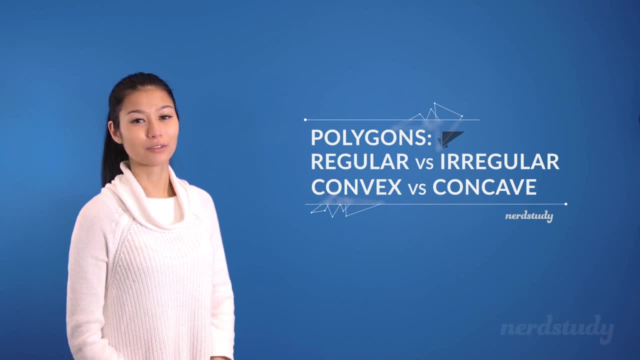 Well, we hope you guys practice identifying what we've learned in this lesson to get a better idea of the characteristics of different polygons. And until next time, have a good one.